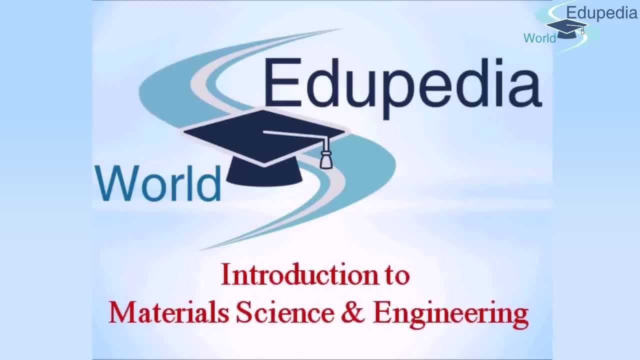 Hi friends, welcome back to the course on introduction to material science and engineering offered by Edupedia World. Previous lecture we saw about crystalline and amorphous materials. We discussed about the different crystal structures and Braville lattice. Today's lecture will focus on three Braville lattice: two belonging to the cubic system and one the hexagonal system. We'll see in details what is. 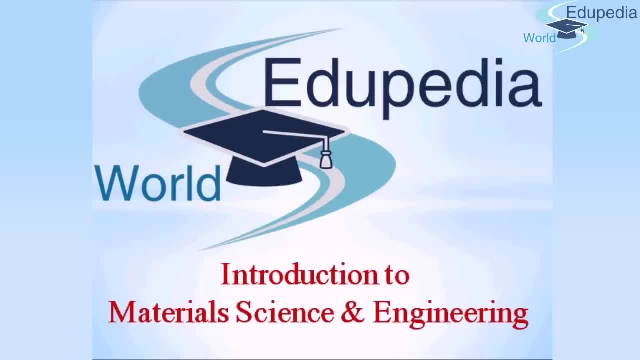 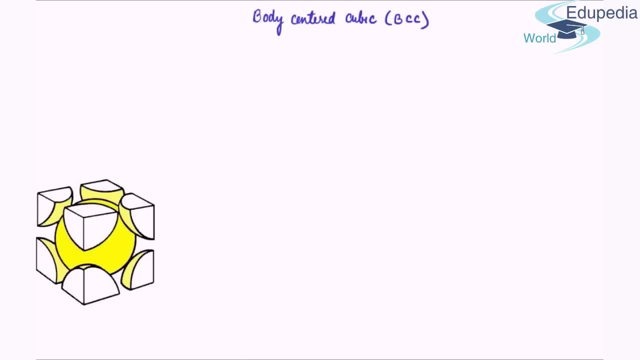 the effective number of atoms in each unit cell for each case, their coordination number, what is the percentage packing and some relevant examples. So let's start our discussion by understanding the body centered cubic system. With our background of crystal systems and Braville lattice obtained in the previous lecture, today's lecture will focus on understanding the cubic system. Why specifically the cubic system? Because 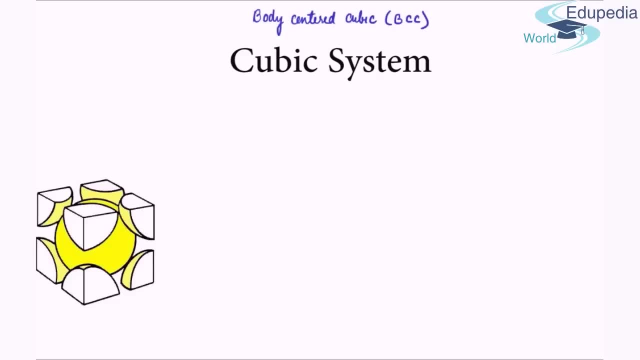 most of the metals have a cubic kind of crystal system. and then we'll also touch upon hexagonal system, because a lot of elements also have hexagonal packing. To begin with, we'll see body centered cubic. To refresh your memory, when talking about a unit cell, what we do is we consider three perpendicular axes and a unit cell is the smallest. 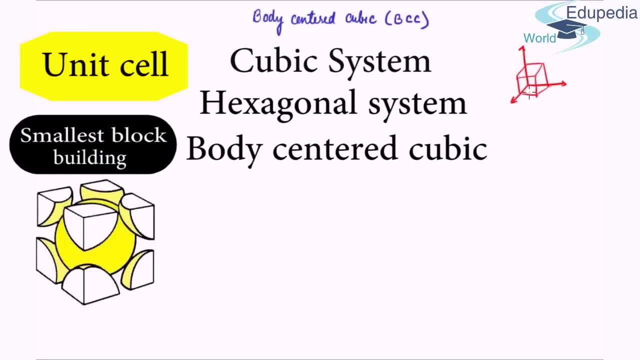 building block, smallest block which can be repeated in three dimensions to get the whole crystal structure. Okay, so this is the unit cell which will be replicated again and again, and again in three dimensions to get the whole material right. So here we'll be discussing with regards to the unit cells. So let's discuss about body centered cubic units. This 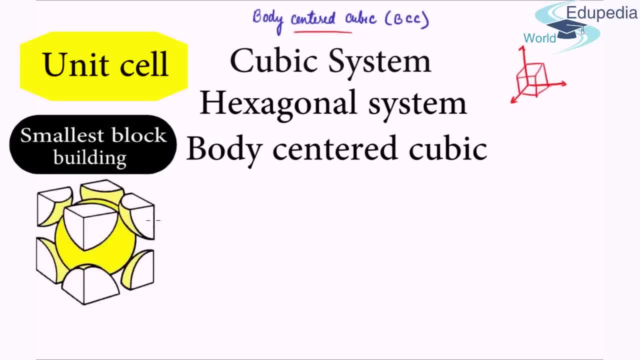 is a body-centered cubic unit cell. So how do we define a cubic system? A cubic system is basically one in which the three dimensions, that is, this length, this length and this length, are equal and the faces are mutually perpendicular to each. that is a cubic system, Now body-centered. 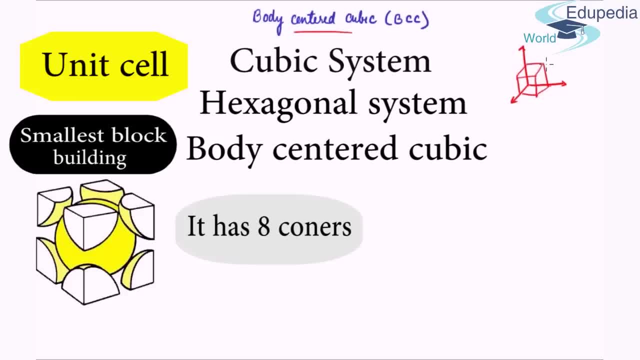 cubic Bravais lattice is one in which the eight corners of the unit cell has an atom each and the center of the unit cell has one atom. Okay, so, as we can see here, one, two, three, four, five, six, seven and one. behind this at the eighth corner, are the eight corner atom and this atom at the center. 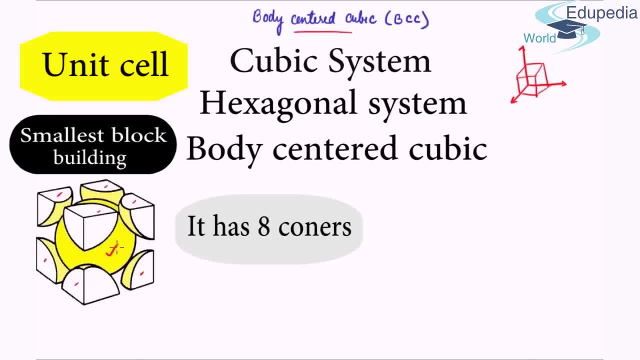 is the body-centered atom, thereby the name body-centered cubic. Okay, now that we have an idea about the specific structure about a body-centered cubic, let us see how many atoms are there in a cubic system. Now, let us see how many atoms are there in a cubic system. 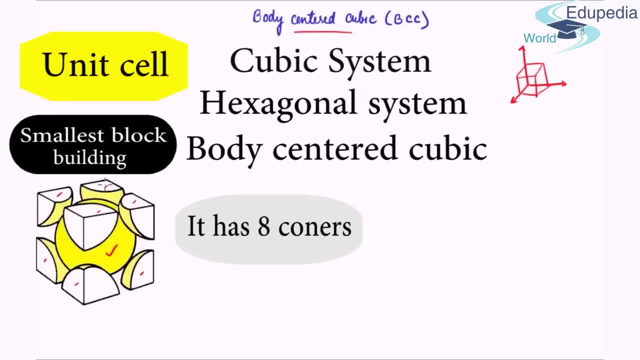 in one unit cell of a body centered cube, as I just mentioned, now that there are eight corners, but each corner atom is shared by multiple unit cells. therefore, the whole atom does not belong to this unit cell. to get an idea about how much of the atom belongs to this unit cell, we need to calculate how many unit cells. 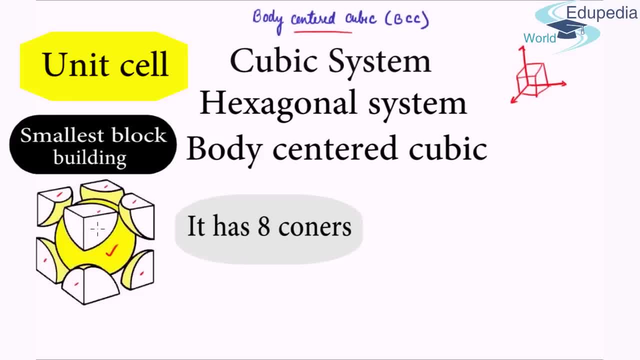 share this particular atom. so let's do that. let's find out how many unit cells share this particular atom. this atom is shared by one, this unit cell itself. second unit cell will be over here to the right of this face, one unit cell will be to the left of this face and one unit cell will be diagonal from here. so 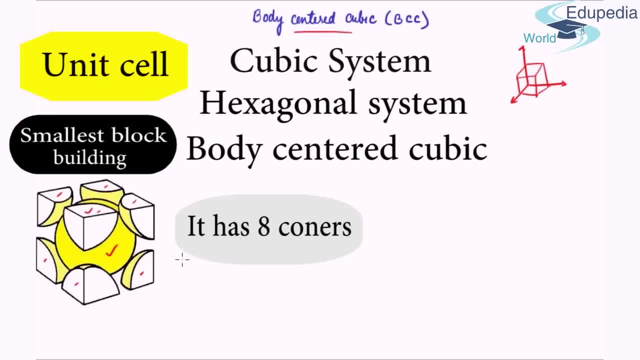 it's like: one block here, one block here, one block here and one block here, making four blocks surrounding this unit cell and similar to this: four blocks in this layer. this is this layer: four unit blocks. there will be four unit blocks just on top of those individual blocks. right, so one layer here, one layer. 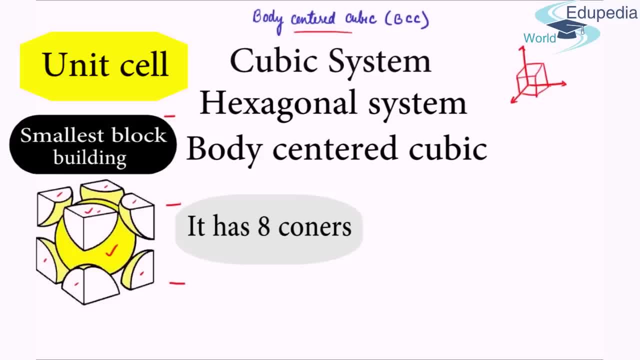 on the right of the face here, one layer on the left of the face here and one diagonal over here. just a replication of this, just one step on top of it. thereby, what we can say is that this atom is shared equally by 8 unit cell. same logic. 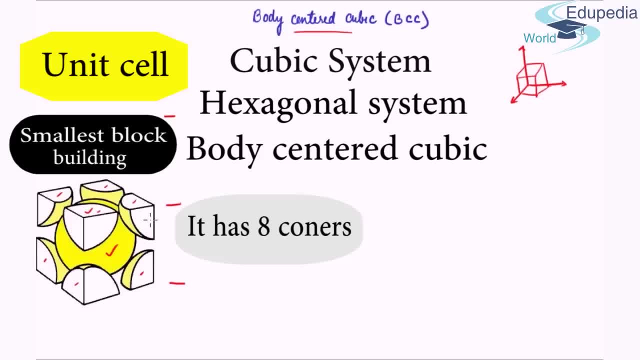 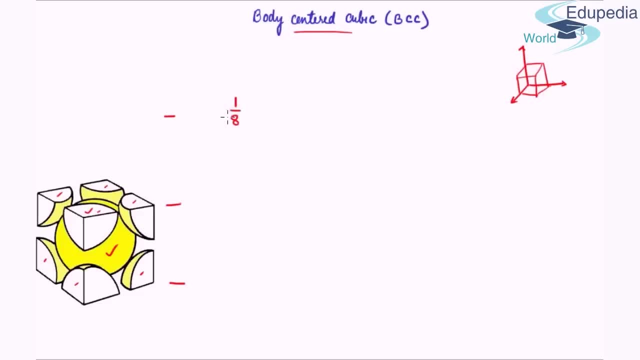 can be imparted to each of the corner atoms. thereby each of the corner atom is shared with the other corner cell by eight atoms. okay, so its contribution, one atoms contribution to this unit cell. this particular unit cell is one upon eight, but there are eight corner atoms. so the effective contribution of 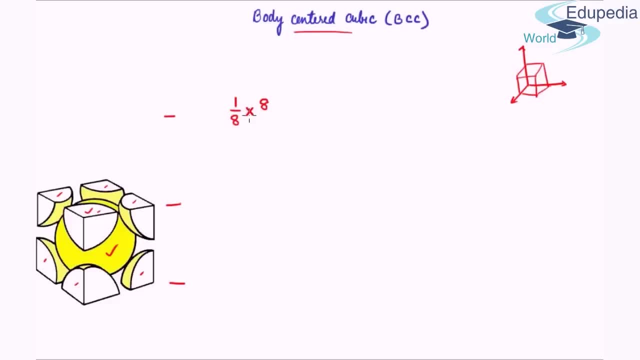 all the corner atoms is one upon eight multiplied by eight. in addition to the corner atoms there is one complete central atom which belongs completely to this unit cell, so one. this gives me two atom per unit cell of a bc. now next thing is: let's understand what is the coordination number. 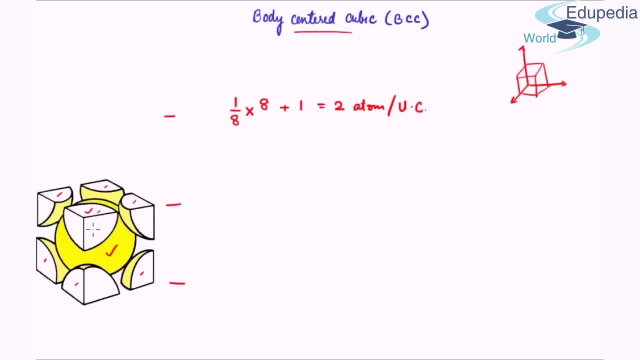 of the bcc atom. before that, what exactly is the coordination? coordination number defines the number of nearest neighbor atoms for a given atom. so the number of nearest neighbors which a particular atom has will be the coordination number of that atom for this body centered structure. if we consider the central atom, there are eight atoms surrounding it at equal distance. 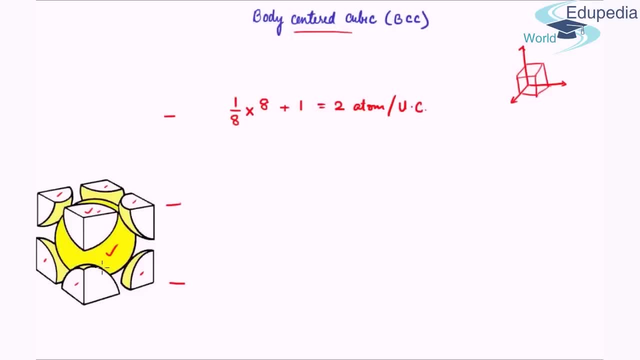 eight corner atoms. therefore, the coordination number for a body centered cubic system is eight. okay, now that we have an idea about how many atoms are there in a unit shell and what is the coordination number number for a body centered cubic, let us find how effectively are the atoms. 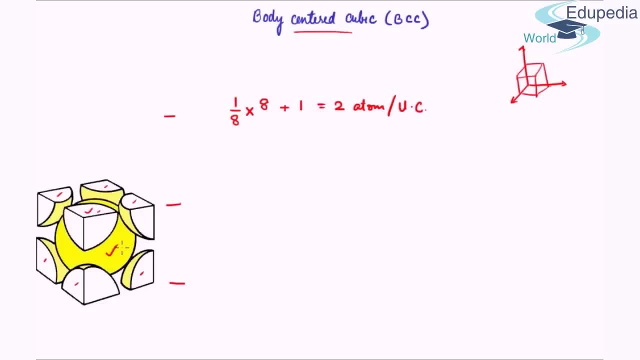 packed in our body, centered, cubic, that is how much space which is available in the unit cell is actually occupied by atoms. this is quite a trivial mathematical formulation. let's do it the side. let me consider it a. if this side is a, all the sides will be a. let's consider the radius of a atom as capital, r, therefore the volume, volume. 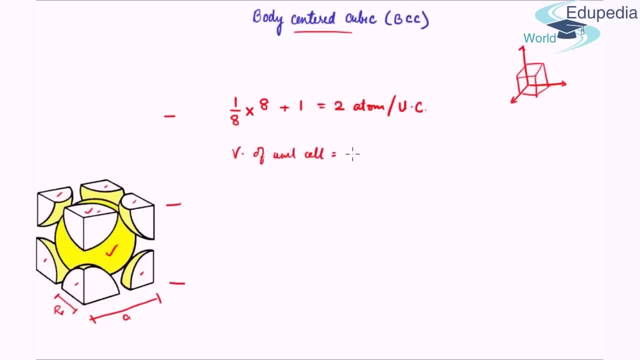 of unit cell. what is the volume of unit cell? is a cube, right, because it's a cube volume of atoms, all the atom, how much there are two atom and each atom is of radius r. each atom will have a volume 4 by 3 pi r cube, which gives me 8 upon 3 pi r cube. now the volume of atoms is in terms of r. 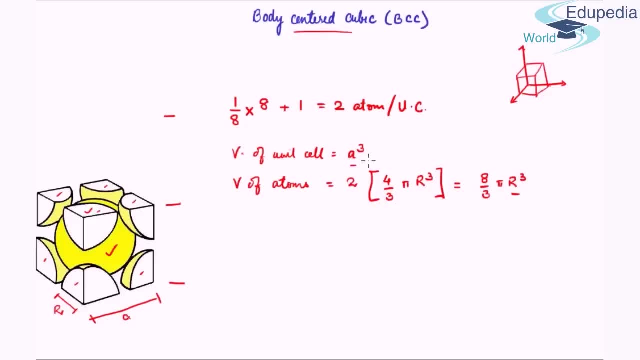 but the volume of unit cell is in terms of a. so we need to find a relation between a and r and using that relation we can turn a cube, something in terms of r and find how much percentage of volume is occupied. but how can we find the relation between a and r? that takes us to 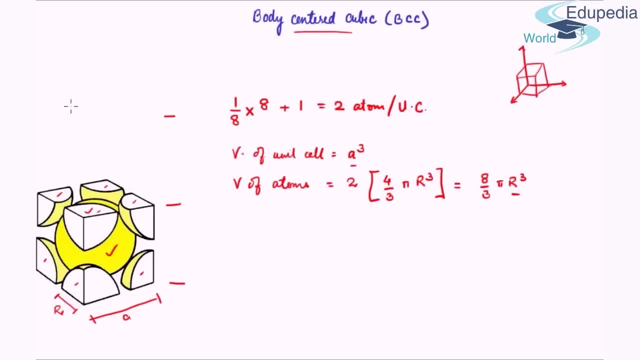 the idea that we need to find the direction in which the atoms are touching each other. is it along the edges? no, because there is a gap along one of the face diagonals. no, because again there will be a gap. what about the body diagonals? what about from here? pardon me, but this should be a straight line from here to here. what? 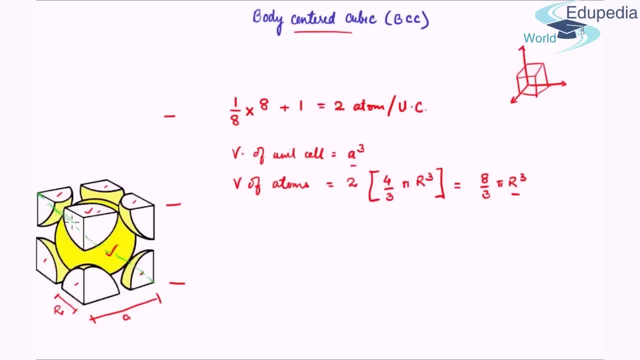 about this. actually, along this direction, the atoms touch each other. this big, this atom touches the corner atom over here and this atom again touches this corner atom over here, so there is a continuity in this direction. now, once we have found out the direction of atoms touching each other, how can we use it to find the relation? 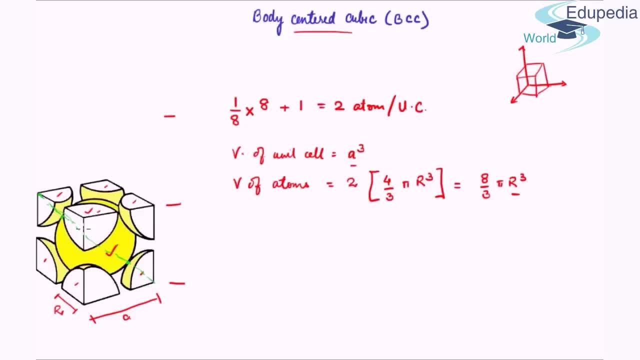 between a and r. we know that this length is root under 3a, right, because this is the diagonal, so root under 3a. but we also know that since the atoms are touching each other, we can find out this length also in terms of r. how come? 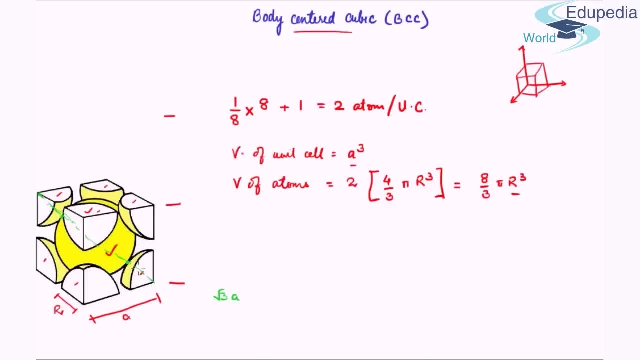 this will be single r, single radius. this is also single radius and this is along the diameter, so two times r. therefore total length is four r. this gives us a relation between a and r. i can write a as four upon root three r, and this i'll replace here. this gives me four upon root three cube r. 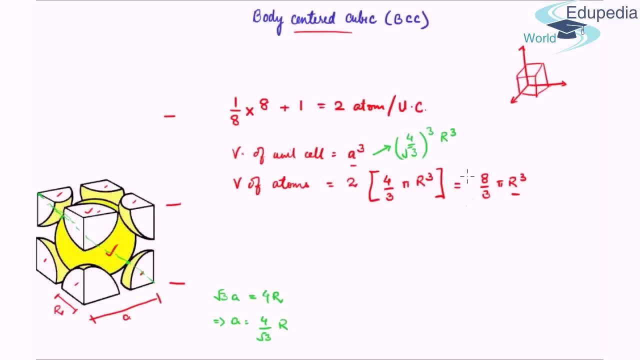 cube. so volume of unit cell, is this volume of atoms, is this percentage packing of atoms obviously is volume occupied by atoms, which is 8 upon 3 pi r cube upon the whole volume of unit cell, which is 4 upon root cube r cube. since it is percentage, we multiply by 100, and this on simplification. 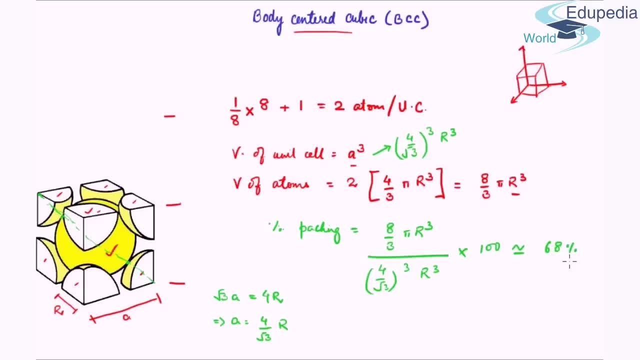 turns out to be around 68 percent. so what we see is a body center cubic structure has 68 percent packing, which means 32 percent of the volume is void right. so does it sound like a good packing fraction? we cannot comment on it for the time being. we need to compare it with other packing. 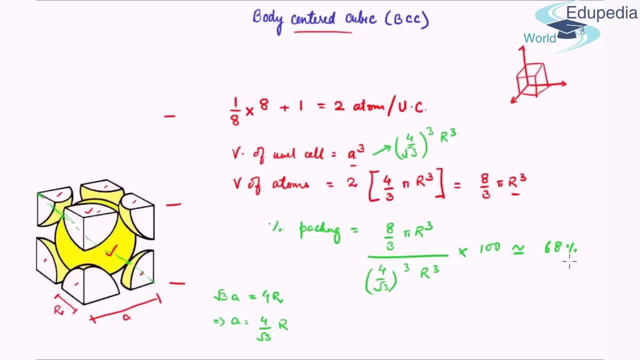 systems and only then we can say how good a packing is. 68 percent packing. right now we have idea about the body centered packing system, the coordination number percentage pack. few examples of atoms and elements which you has body centered cubic packing. the most prominent one is iron at room temperature, in addition to 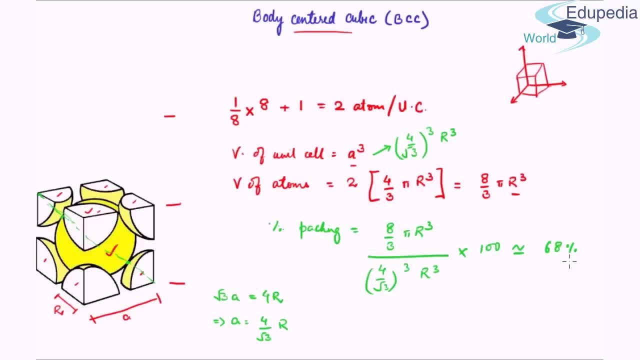 that we have tungsten molybdenum potash. these all are examples of body centered cubic packing. right now, with the background of body centered cubic, let's next see the face centered cubic system. face centered cubic system also belongs to the cubic crystal system, so 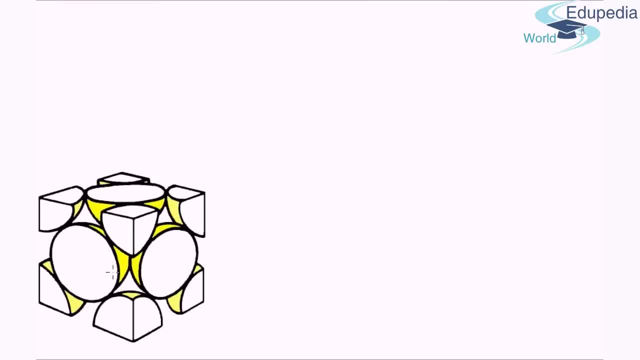 the sides will be. sides will be of equal length and the faces will be mutually perpendicular to each other, as in this case of body centered cubic. the difference will be: in body centered cubic you had a atom at the center, body center and eight atoms at the corner in the fcc, or the face centered cubic. 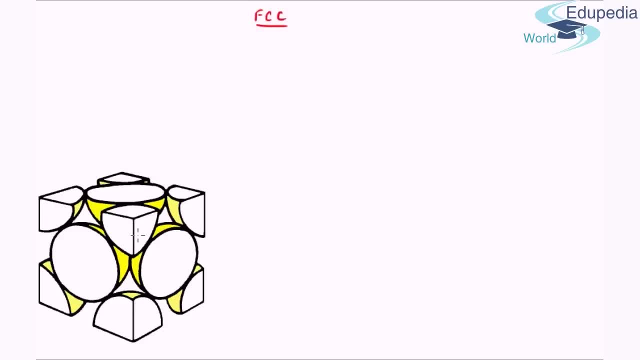 we have eight atoms at the eight corners, same as the body centered, but we have six atoms at the six faces. to make a cube will require six faces right and each face center will have one atom. so the six faces: one here over here, three: one at this face over something over here, one at the back face over here and one at 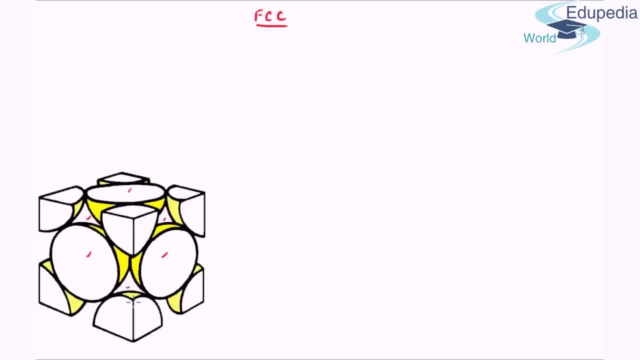 the bottom face somewhere over here. so those six face centers, six atoms, eight corners. obviously eight atoms result in the number of effective atoms, that will 103 problems. the number of effective atoms has the entity which can only Along with the impact We have seen. the number of effective atoms in a body centered system was 2.. 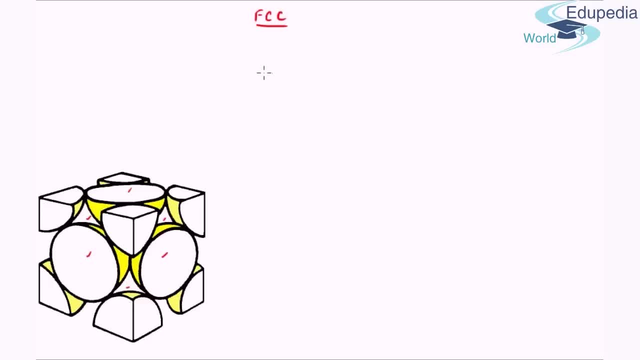 Let's calculate the same for the face centered system. The corner calculation will be same: 1 upon 8 multiplied by 8, because it is practically the same thing. But what is the contribution of the face centered atoms? Let us consider this particular atom. 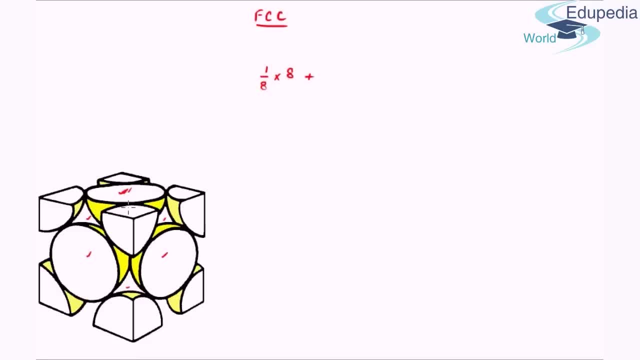 This is shared by the unit cell at hand and the unit cell just above it. So every face centered atom is shared by two units and we have six face centers. So contribution of each atom to this particular unit cell is 1 by 2 and we have, effectively, 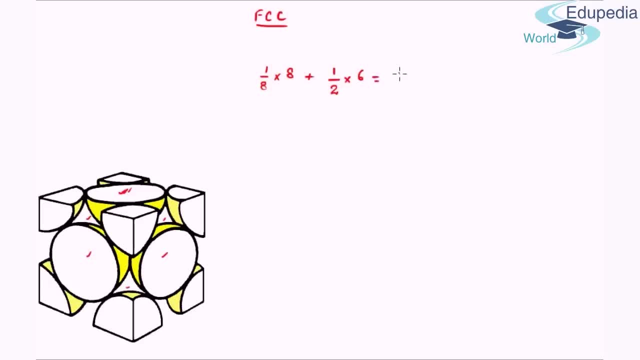 six faces. So times six, This gives us four atoms per unit cell. Okay, This is my number of atoms per unit cell. Next up, what will be the coordination number for the FCC, For the BCC? you could easily visualize it. 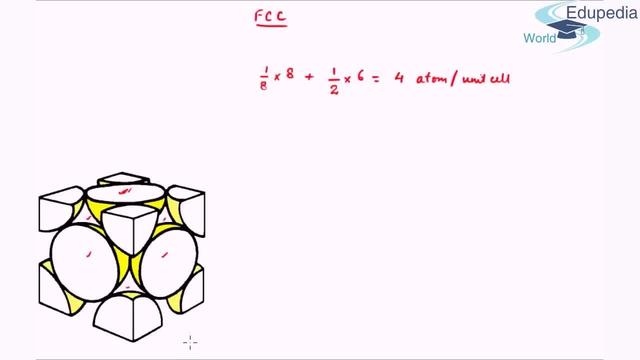 It was 8.. For FCC, take my word, for the time being it will be 12.. But I will explain it with a much easier to comprehend diagram in a couple of minutes. Before that, let's understand the packing fraction of the FCC. 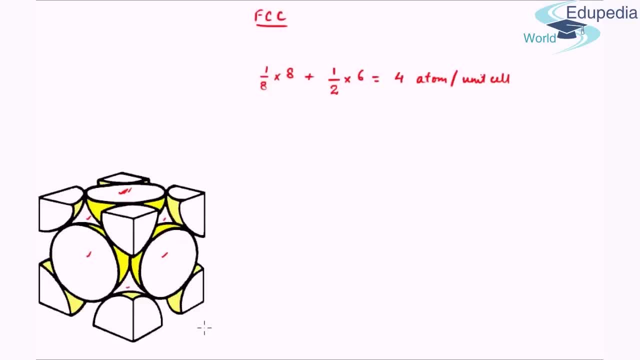 Is it better than BCC? worse than BCC? If better, how much better? Let's do the calculation This side again. let's call it A The radius, let's call it R, So the volume of U is equal. 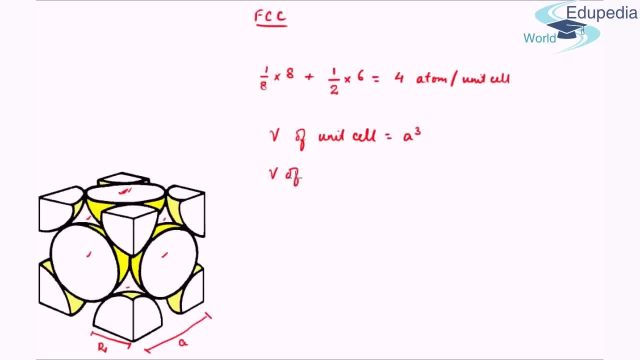 to unit cell again be A cube. Volume of atoms in the unit cell we have four atoms, So four times volume of each atom is 4 upon 3 pi R cube. That gives us pi upon R cube as the volume of all the atoms in the unit cell. 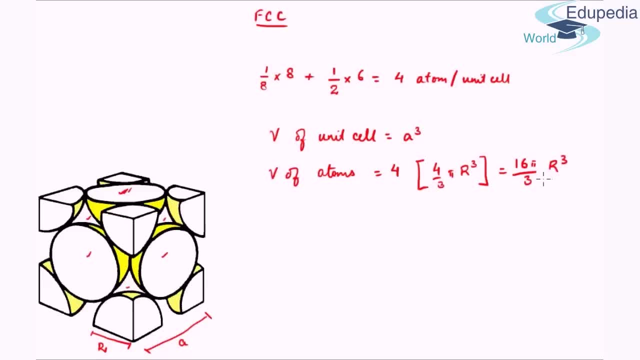 Again, we need to find the relation between A and R to calculate the packing fraction. Now, which is the close packed direction? Is it this direction? No, there is a gap. Is it this direction? As it turns out, actually, the face diagonal is the close packed direction right. 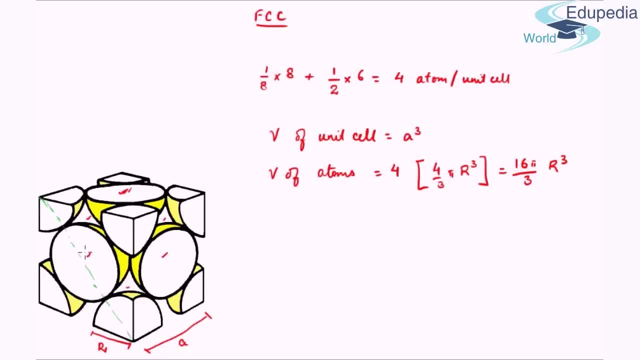 So let me draw it here. So this is the close packed direction, the atoms touching each other here and here. Therefore, this direction length will give me the relation between A and R. Let me make that calculation. This length is root under 2A and again there are length R, length 2R and length R, which 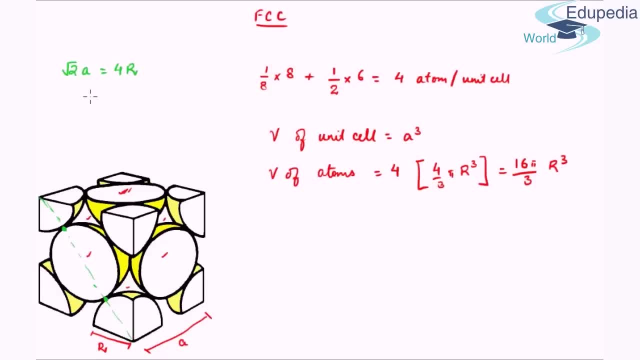 is 4R, So root under 2A is 4 times R, which gives A is equal to 2 root under 2R. I will plug this over here. This gives 2 root under 2 cube, R cube. Thereby the percentage packing. percentage packing is volume of the four atoms upon the. 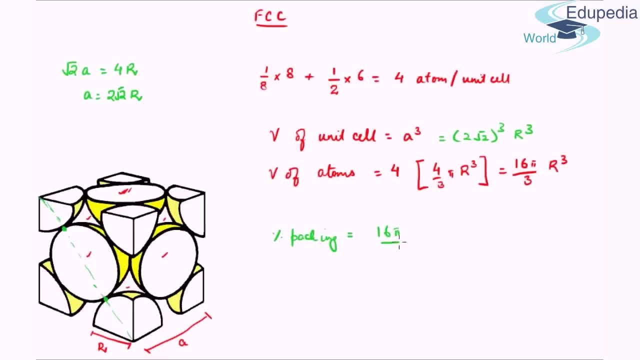 volume of unit cell, which is 16 pi upon 3 R cube divided by 2 root 2 cube R cube multiplied by 100. And this approximate to 74% if you calculate it. approximately 74% packing in the case of face centered cubic. 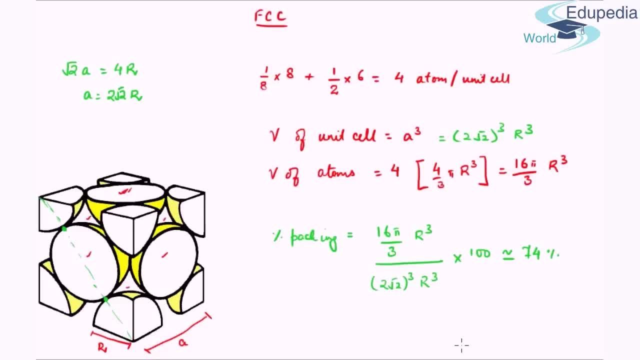 So we see that the packing fraction is marginally better than body centered. In fact it is 6% better, but still there is 26% void present in face centered cubic. So what we can say is: body centered cubic is not very dense packed. 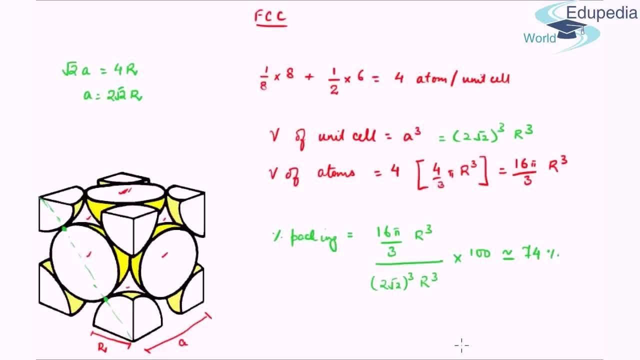 Face centered cubic is better packed than body centered cubic, but still there are a lot of voids left. Now, as we will see in future lectures, this voids, this void spaces which is present due to ineffective packing, will come in quite handy while alloying. 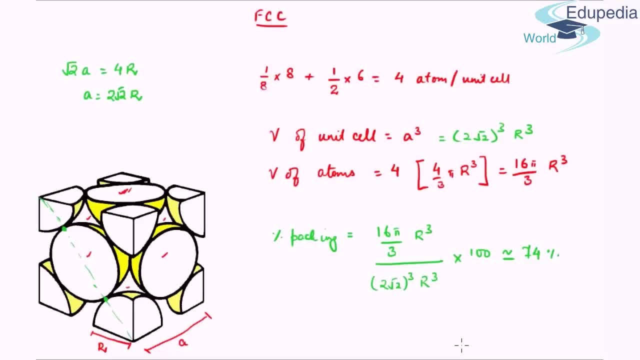 These are the places where atoms will go and reside in case of alloying with small atom. We put that thought into hold for the later lecture. Now The important elements which has face centered cubic packing are copper, aluminum, nickel, silver. These are face centered cubic atoms. 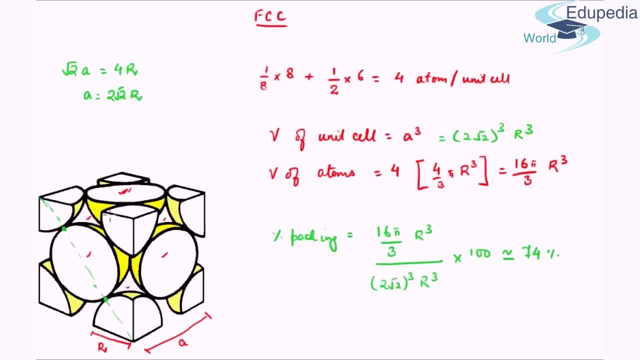 Now this representation over here. I said that the coordination number is 12 for FCC, but it's quite difficult to comprehend from here. In order to give you a much clearer visual perspective about this, let me handle the question in a different way. 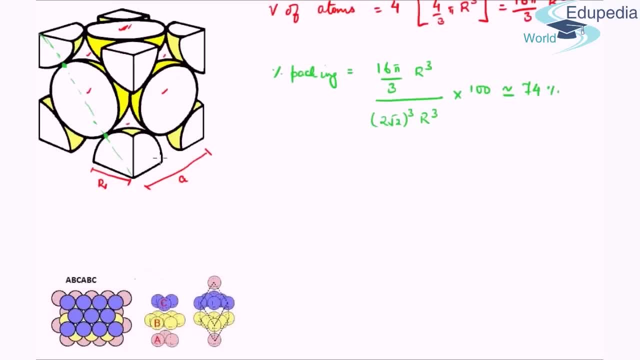 And let's show you a different diagram. Okay, so this is what is known as a ABC-ABC type of structure. ABC-ABC, Whenever you hear the term ABC-ABC packing. This is also an alternative reference to the FCC type of packing. 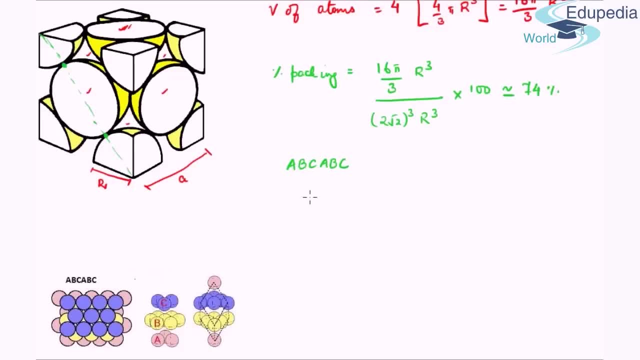 They both are synonymous, It is just a different way of representation. Now let me give you an idea about what is ABC-ABC packing or ABC-ABC stacking. So here we have shown three layers. The pink layer is the bottom layer. The blue layer is the bottom layer. 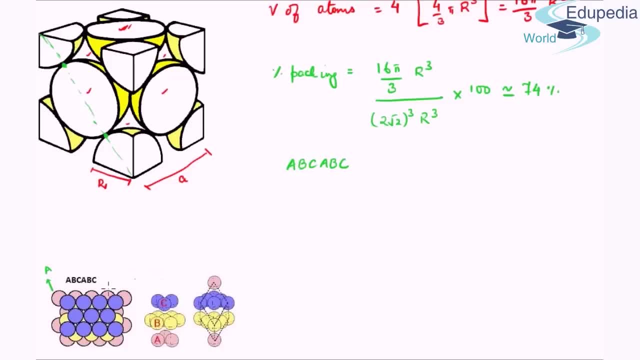 This is layer A. The yellow layer is the middle layer, which is the layer B, And the blue layer is the top layer, which is layer C. Now if I say I give you marbles of equal radius and I say you keep one marble and try to surround it with maximum number of marbles in the same 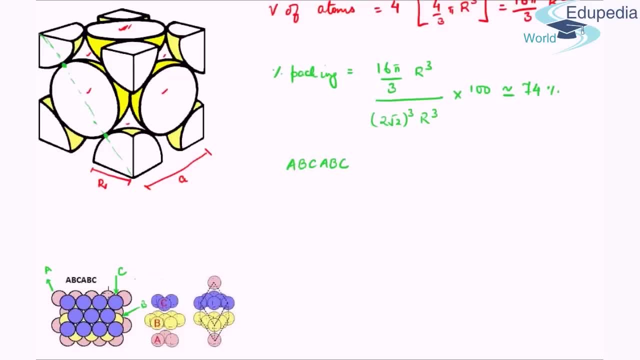 plane. How many marbles do you think you can surround it with? In fact, what you'll find out is that a single marble Can be surrounded by a maximum of six equally sized marbles in the same plane that is shown over here. 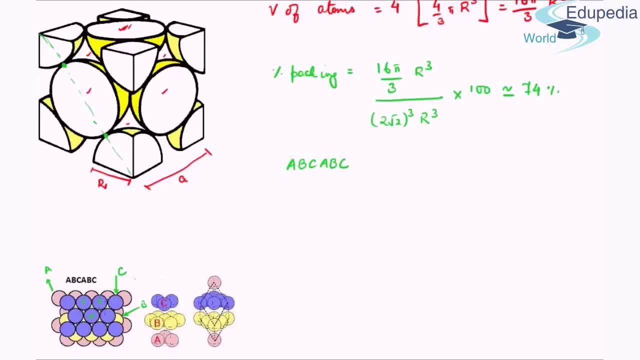 If you consider this particular marble, then one, two, three, four, five, six. this six marbles will complete the packing surrounding this central marble and that is packed to maximum density. Okay, And when you see in such packing, you will see observe. 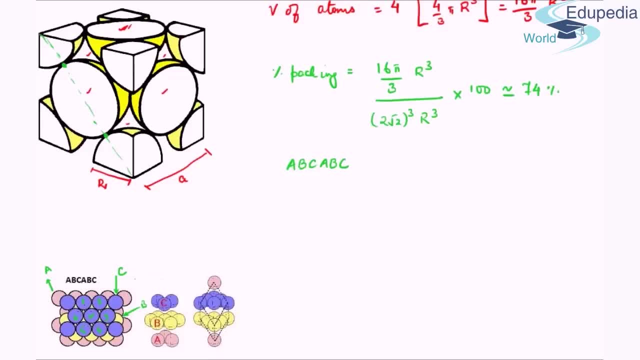 There are voids left right, There is void here, void here, And the void comes in two categories. One, let's say, will be something like this: a triangle pointed upward, And another, you will see, is like this, a triangle pointed down. 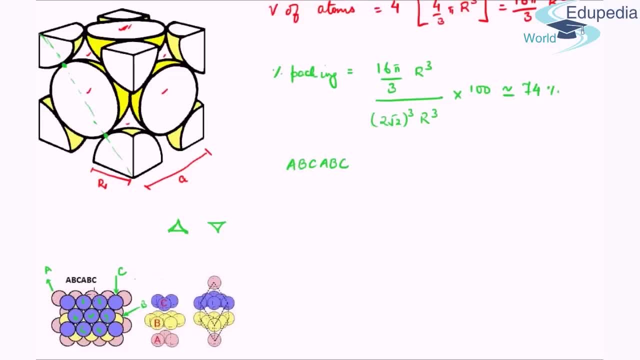 Okay, Now let's say that the first layer is also similar to the third layer, right? So you can use this to visualize the first layer, though we have some layers sitting on top of the first layer. You can, You can use this to visualize first. 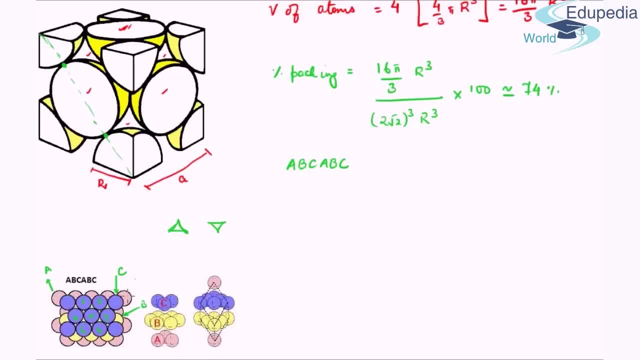 So once I lay down the foundation or the layer A over here, I will have two options: either this type of hollow or this type of hollow to fill the second layer. Let's, for the sake of argument, say that I picked up this type of hollow to fill the. 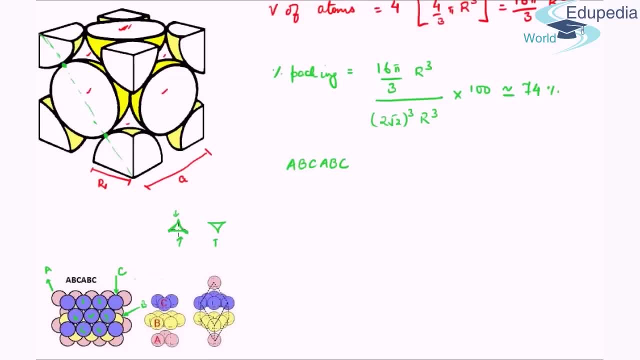 second layer. I filled out the second layer. Now I will again have this type of hollow leftover or the hollow sitting right on top of the base layer or the A layer. Okay, So if I go again on top of the A layer for the third layer, then what we get is known. 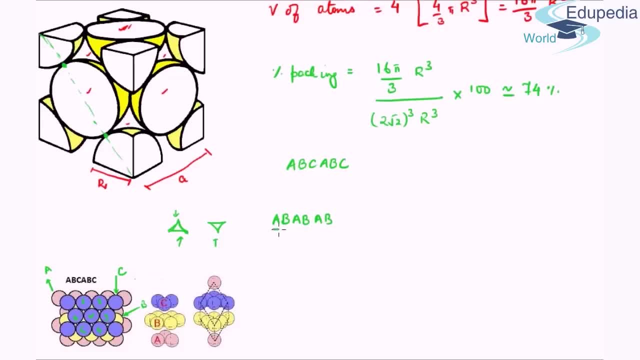 as AB, AB, AB packing. That is first layer, upper triangle hollow. Then again first layer, upper triangle hollow. first layer, upper triangle hollow. But if we go like this, you lay down the first layer for the second layer, you go for this. 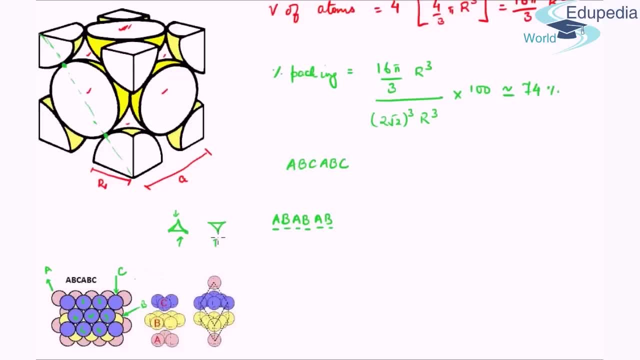 hollow. Third layer. you go for the other side, sided void- Then what you get is ABC, ABC kind of packing. You have three distinct layers. Okay, So this is my FCC kind of packing, As we'll see in later discussion. if we go by AB, AB, AB kind of packing, then what we get 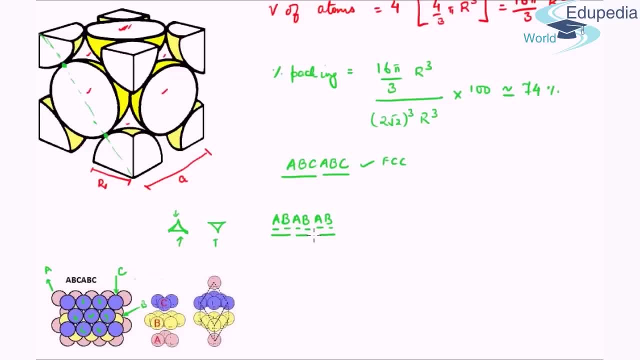 is hexagonal packing, But let's stick to ABC, ABC packing. Now suppose I visualize this from the side, from here. If I see this, then what I will see is a layer- bottom layer like this, a middle layer like this and a top layer like this. 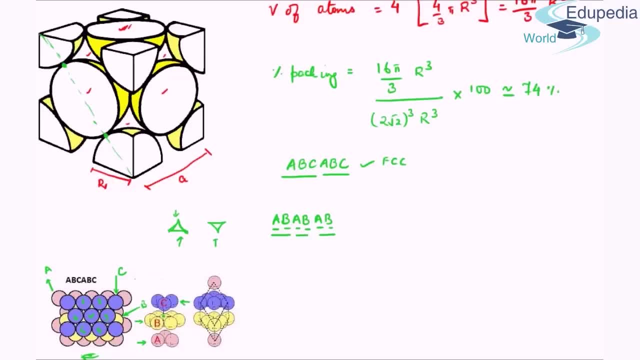 This is what you will visualize And if you consider this particular atom, this atom will have six atoms surrounding it in its own layer, three atoms surrounding it on top of it and three atoms surrounding it from bottom. Therefore, this particular atom has 12 atoms surrounding it, which means its coordination. 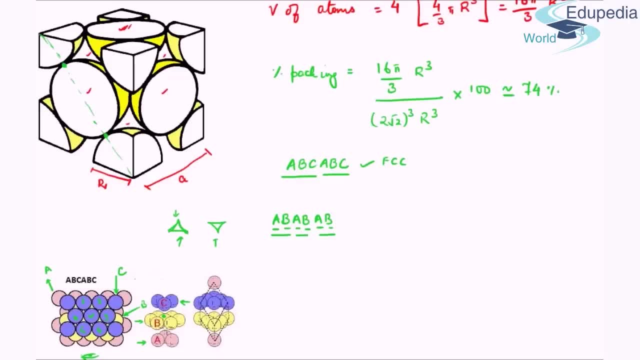 number is 12. Isn't it? That is the basic definition of coordination number. Now this? there's nothing special about this atom, right? This is a randomly picked atom. Okay, This is a random pick up from the whole set of atoms. 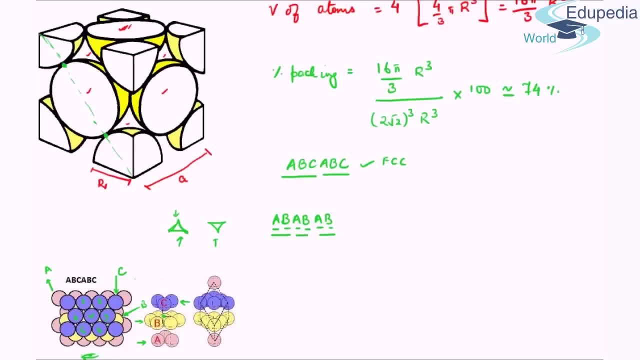 Therefore, if the coordination number of this atom is 12, then the coordination number of any atom in a FCC kind of system will be 12.. Therefore, what I can say is the coordination number for FCC system is 12.. Okay, I hope this is clear. 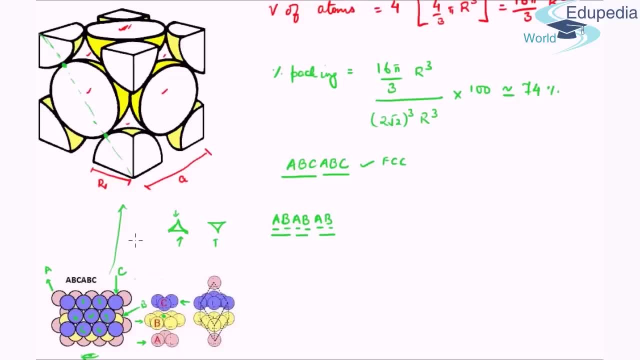 Now, how can I visualize this, turning into this Quite tricky right? Let's help you out. Let's imagine just one atom from here, One atom, any one atom, and just the top three atom and additional three atoms sitting like this. So six atoms in total, then six atoms in total, sitting in the opposite direction, the opposite. 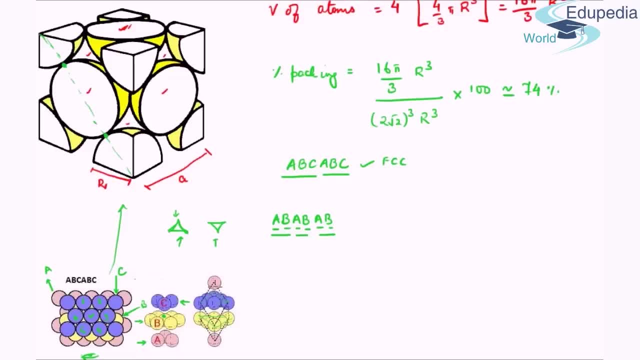 triangle and one atom, just the mirror image, two layers further upwards right And then if you try to join and form the cube, you can see that this is actually a segment of the face centered cubic. So If you take out some time and try to visualize this, you can actually see how this turns. 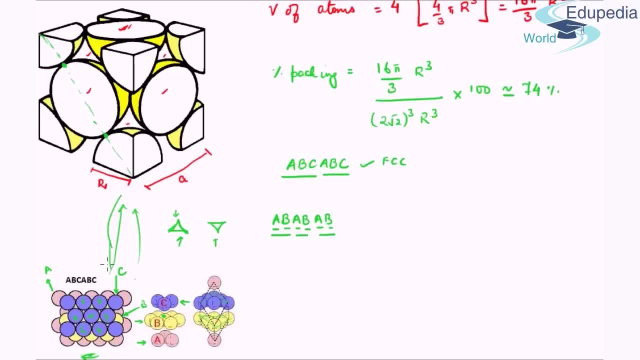 into this or vice versa, how this turns back to this. But the take home from the discussion here is: FCC is one of the most important kind of crystal structure, which has a 74% packing. has 12 as its coordination number, alternatively, 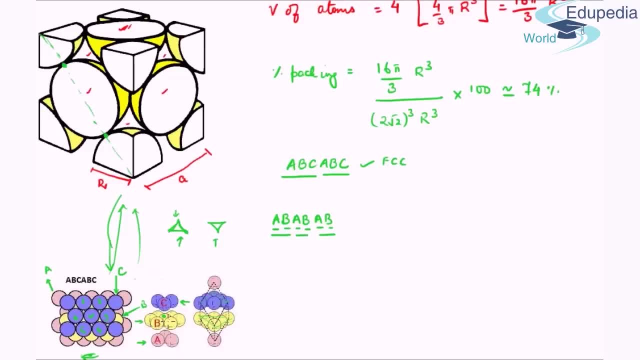 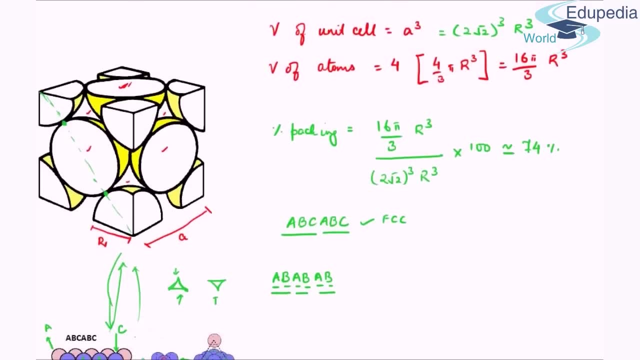 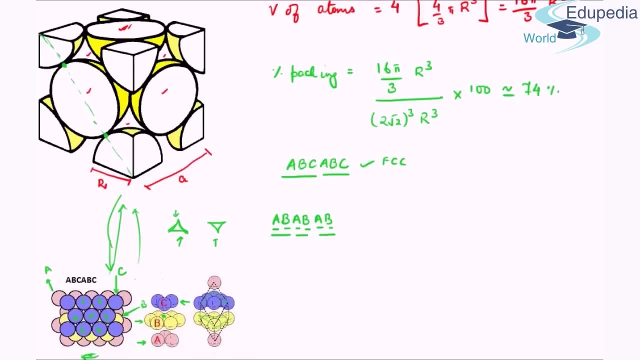 known as the ABC ABC kind of stacking, because it has three distinct layers repeating each time, And the packing fraction is better than in the case of BCC right. This closes the crystal system for the cubic system. Let's jump into the hexagonal system and try to understand that. 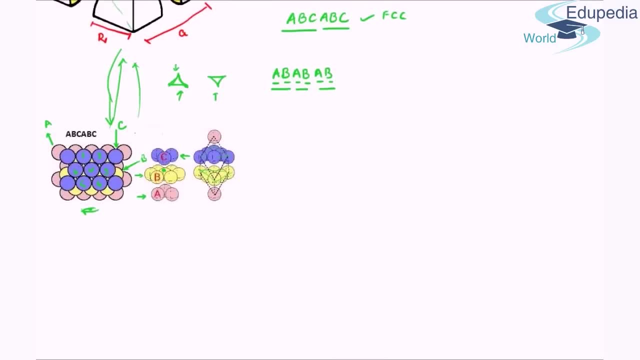 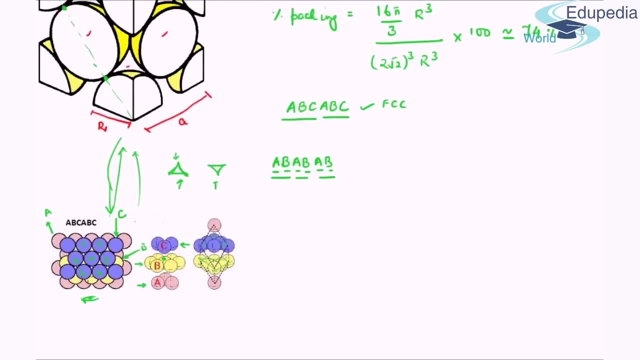 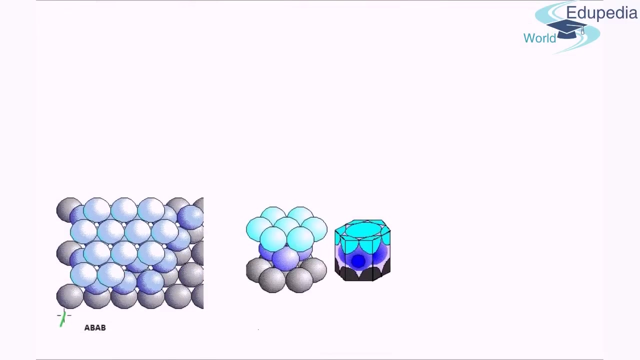 As I have already mentioned here, the hexagonal system is quite similar to the face centered cubic, in the sense that the basic foundation of atoms, the arrangement of items, is the same, Just the repetition is different. So let me show you here. Here you can see, is this is my A layer and this is the B layer. 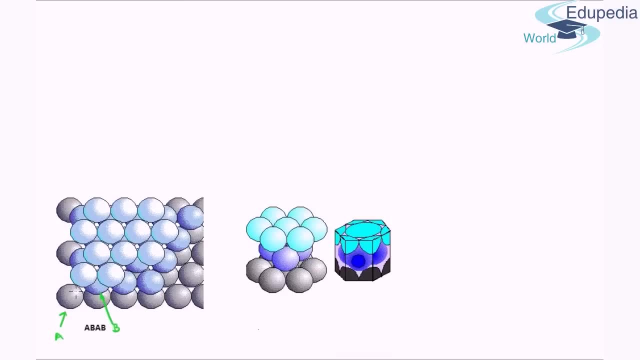 Okay, And the third layer is again the A layer. So another atom here, atom here. So this atom beneath that in the first layer was also an atom over there. And the fourth layer will again will be an atom over here, an atom over here. 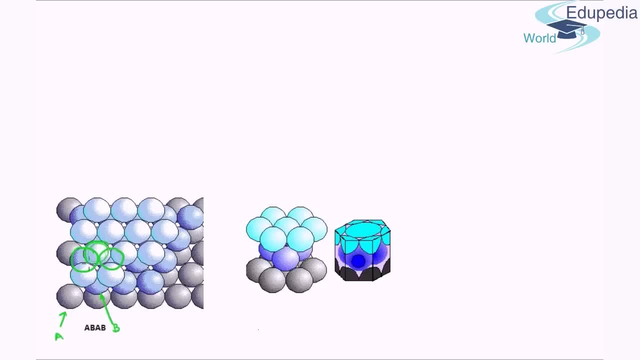 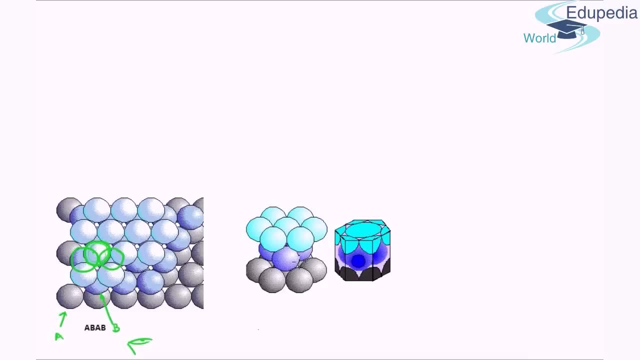 that the bottom layer: one atom at the center and six surrounding it, then three atoms like this on top of that And again the bottom layer, repeating it Right. So what you can see is this: alternatively can be shown over here Is: 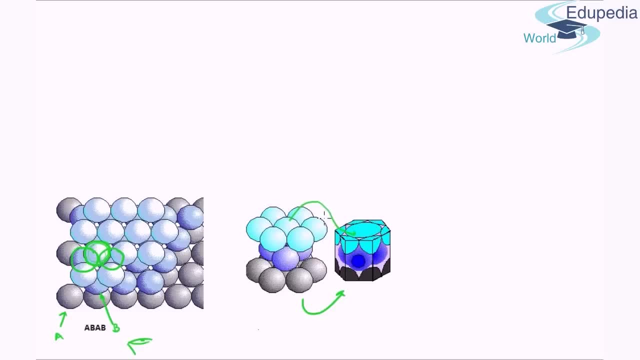 Something like this: with the central atom, six atoms at the six corners, three central atoms here And again the six atoms with one central atom over there. So this gives you the hexagonal packing. Now for the hexagonal packing. what is the coordination number? again, 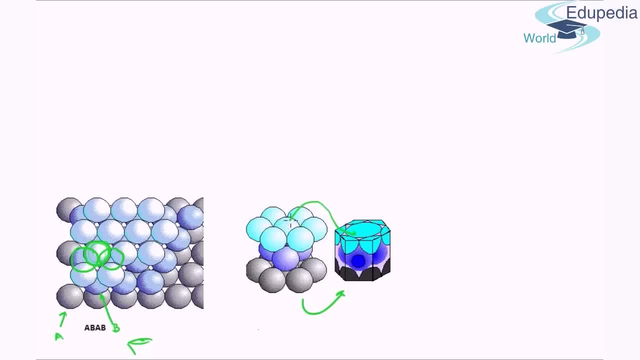 You can again think of it in the same way as the FCC. So if you take this atom, six atoms here, three atoms at the bottom, three atoms will be at the top. So for the hexagonal packing system also There will be the coordination number of 12.. 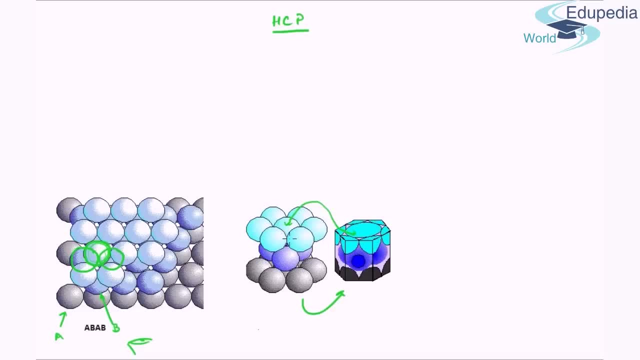 What will the packing fraction? a similar argument to that of the FCC can be given and said that HCP will also be 74%. Why? Because the packing system or the basic packing pattern is the same, Only the stacking stacking sequence is different. 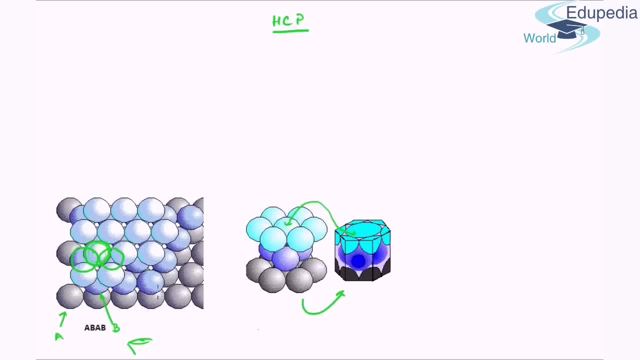 In FCC it was ABC, ABC. Here it is AB, AB. But each layer in itself is packed as compactly As possible And the second layer is placed on top of first layer as compactly as possible. Same as in the case of FCC. 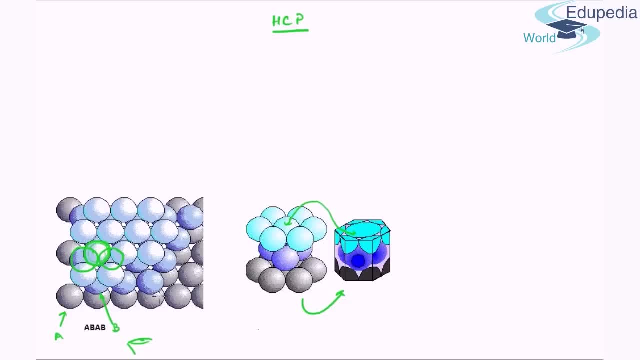 So even here, the packing fraction is 74%. Okay. Now, uh, interesting idea is that if this is a okay, then this high can be calculated as 1.6,, 3,, 3, a fight. Some of the examples of hexagonal packing is one of the most prominent is magnesium. 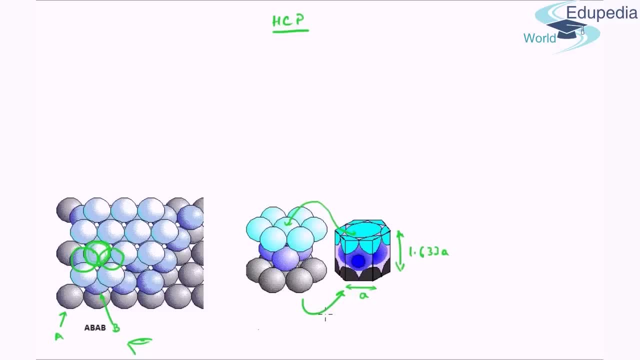 Okay, Then we have uh, others like cadmium zinc and uh zirconium. such elements are belong to the hexagonal packing Now, in fact, the hexagonal packing system shown here is not the unit cell. This is not the unit cell. 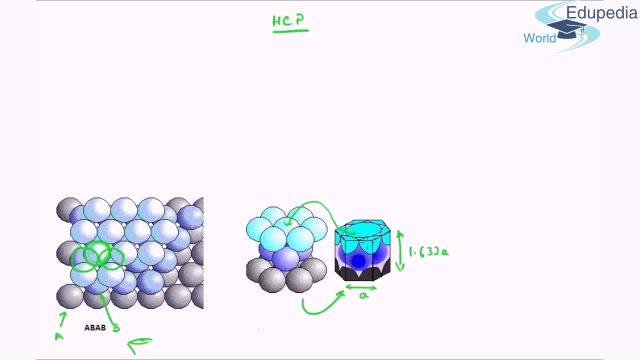 This is basically made from three unit cells. Okay, With each unit cell following the criteria: A is equal to B, is not equal to C, And And angle A equal to angle B, equal to 90 degree, but angle C is equal to 120 degree. 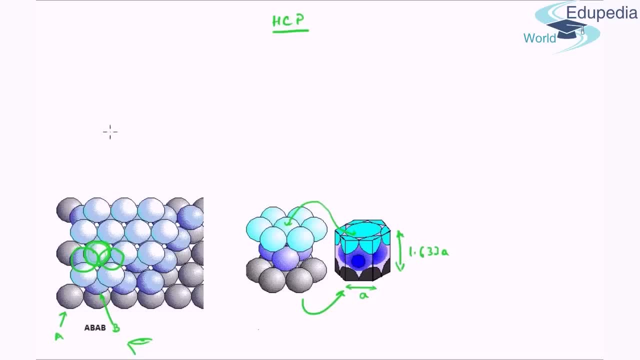 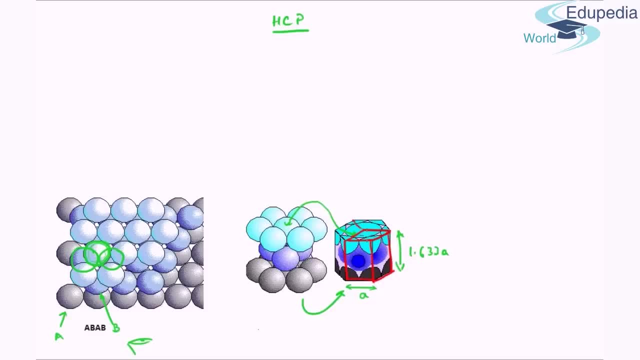